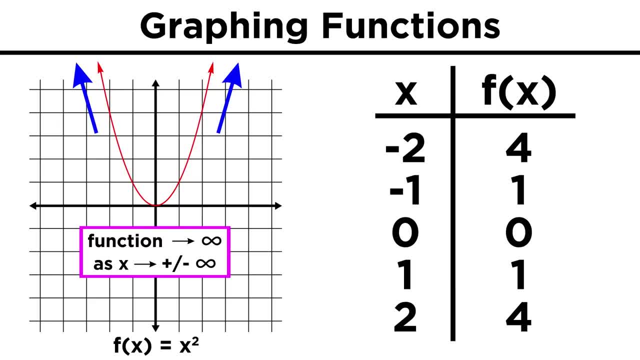 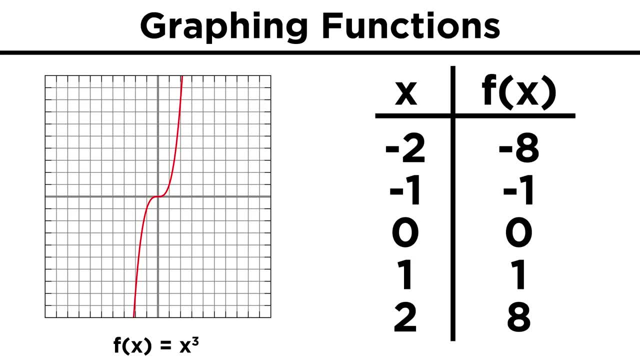 negative or positive infinity. We can look at what even higher degree functions do as well. Here is x cubed, Now the function grows even faster. but we must note that when we cube negative numbers, we get negative numbers. so as x goes to negative infinity, the function goes to negative infinity. 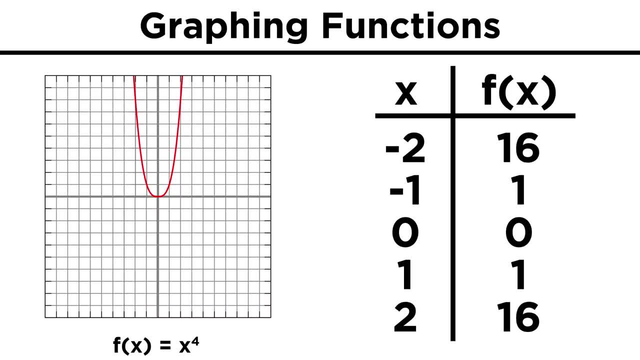 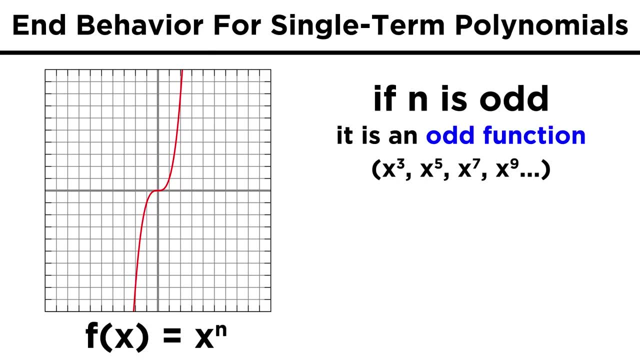 rather than positive infinity. If we look at x to the fourth, it goes back to looking like x, squared, just steeper. In this way we can make the generalization that for a polynomial with one term, if that term has an odd exponent, it is an odd function and it will somewhat resemble the x cubed. 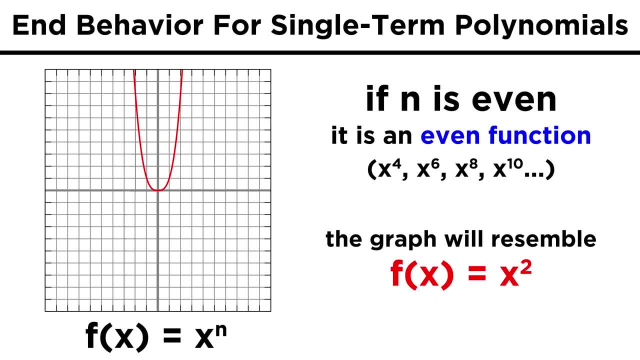 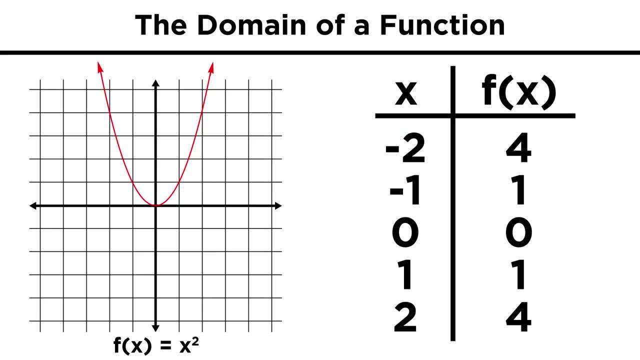 function. If the exponent is even, it is an even function and it will somewhat resemble the x squared function. Another thing we must frequently describe is the domain of a function. As we mentioned before, this is the set of all the functions that are related to the 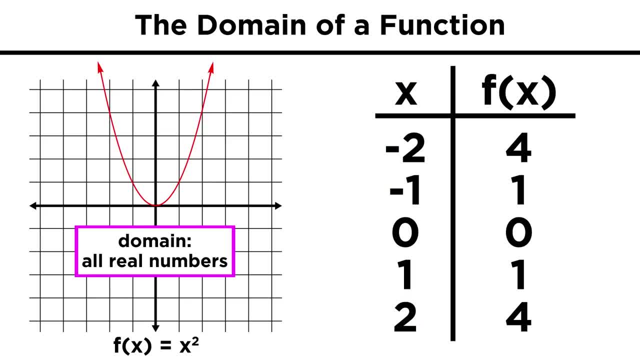 domain of a function. The domain of a function is a set of all allowed x values. Very frequently, the domain will be all real numbers. This is because for most lines and curves, any x value can be plugged in, and we can see this represented visually with a graph that extends infinitely in both horizontal. 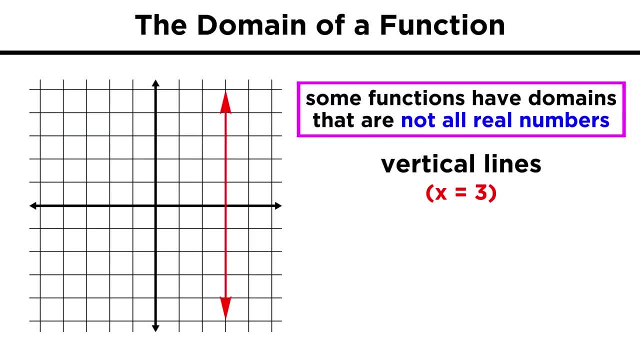 directions. Exceptions would be things like a vertical line. Here only one x value is in the domain. There are also instances where a sum or difference in the domain is not represented. This is because for most lines and curves any x value can be plugged in, and we can. 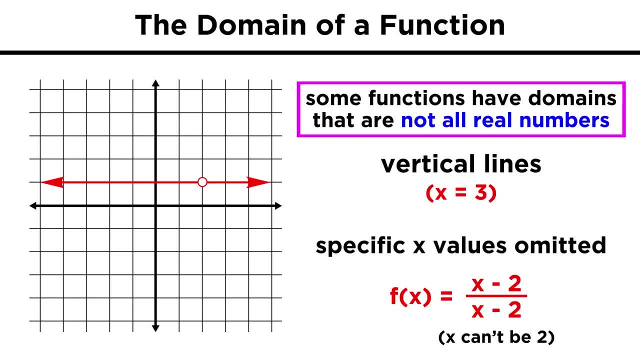 see this represented visually with a graph that extends infinitely, in both horizontal directions, The set of all the functions that are even. it is an even function. The domain of a function rules out a specific x value so as to avoid dividing by zero, as 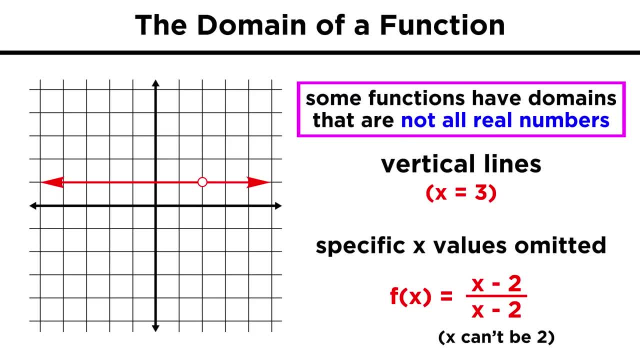 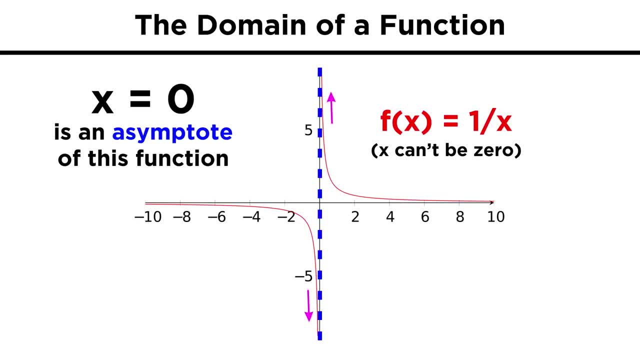 this would produce undefined values. This is where we get asymptotes whereby a value is missing from the domain and the function will typically go towards positive or negative infinity as it approaches this missing value. More on those later. By contrast, the range of a function or the set of all the functions that are related,